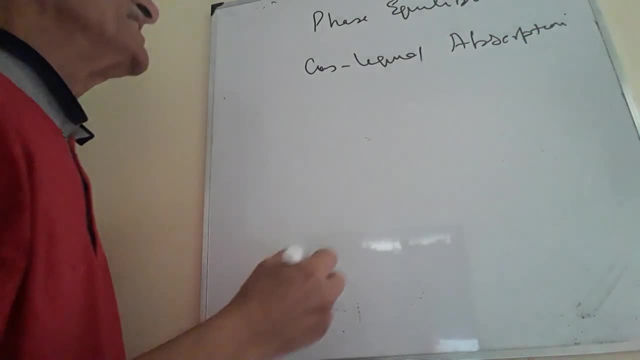 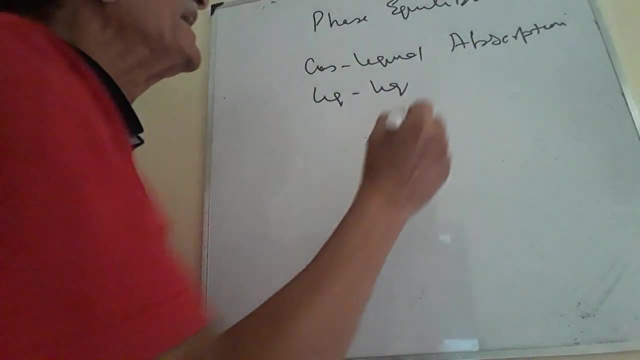 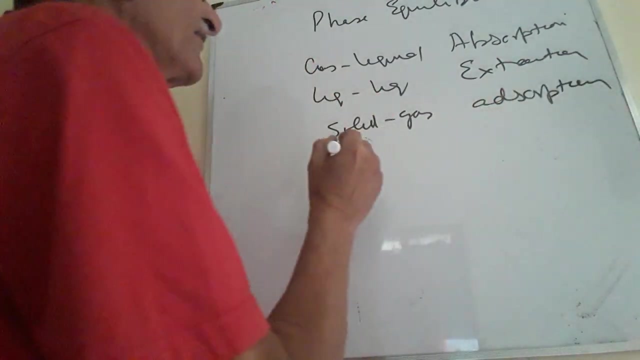 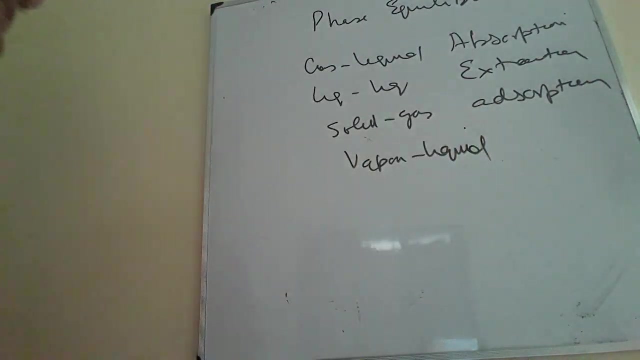 You can pass hydrogen gas to the oil. That is absorption. Then liquid-liquid. It is called extraction Liquid-liquid. Yeah, Extraction Solid-gas absorption, Absorption Vapor-liquid, Vapor-liquid, Phase-liquid. 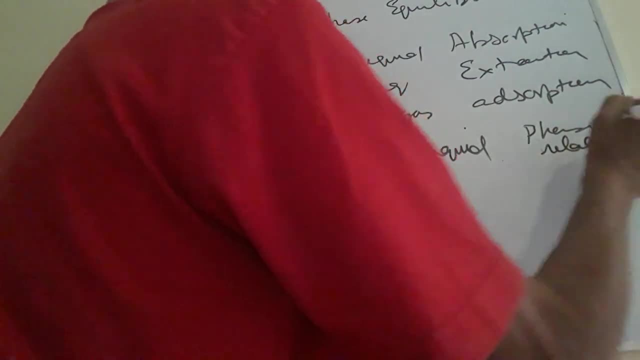 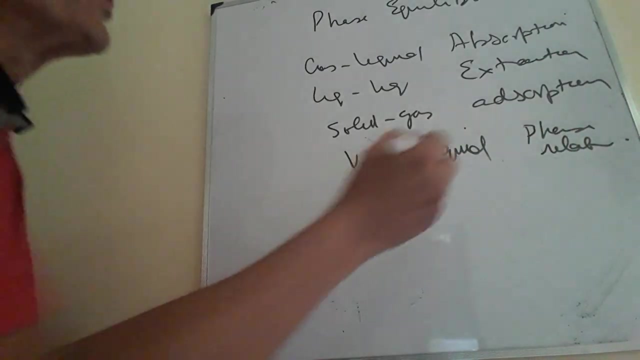 Phase-liquid, Phase-liquid. Now, this is elaboration Phase-liquid. This is what you are using in distillation. Distillation- Vapor-liquid is called distillation. Okay, So we are going to concentrate on vapor-liquid equilibrium, because in many petrochemical industries it is very common. in chemical engineering, vapor-liquid equilibrium is very, very important. 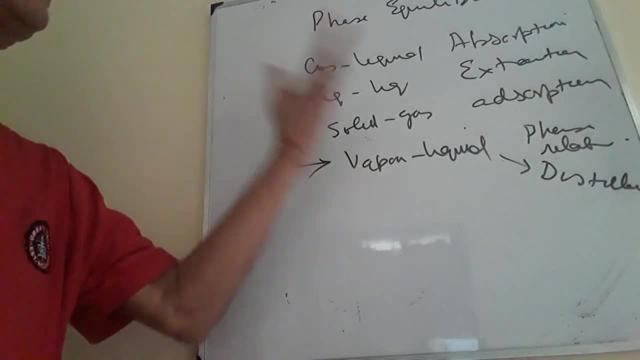 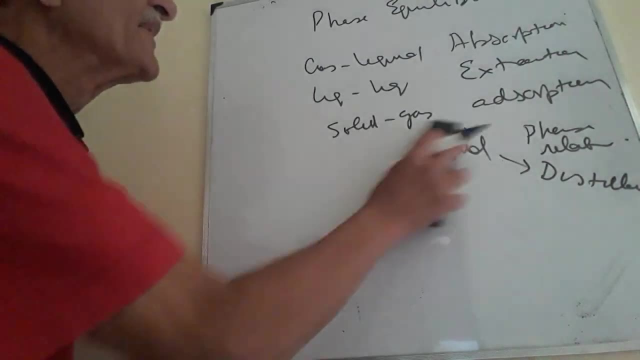 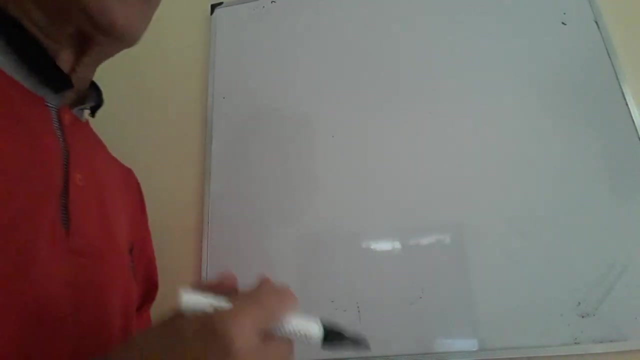 So I am going to take the vapor-liquid equilibrium and try to study that thoroughly. Of this gas-liquid, liquid-liquid, solid-liquid-gas you can study elsewhere. Now for equilibrium, for example, if you have got mechanical equilibrium pressure on the system and surrounding, 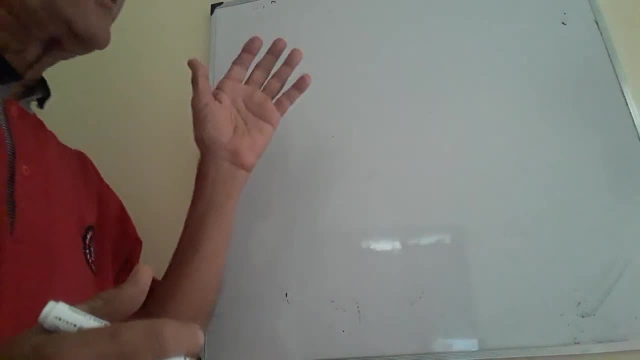 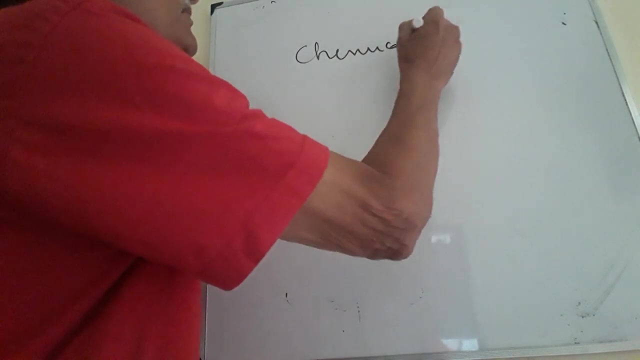 it will be same. Simply, thermal equilibrium means temperature of the system and surrounding will be same. Now we have got what is called as chemical equilibrium. Chemical equilibrium, Now. chemical equilibrium Now. how are you going to define chemical equilibrium? 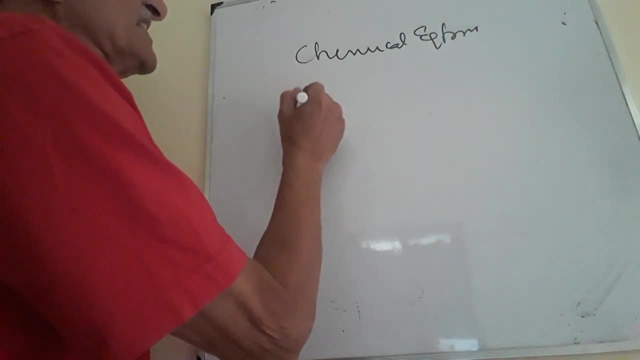 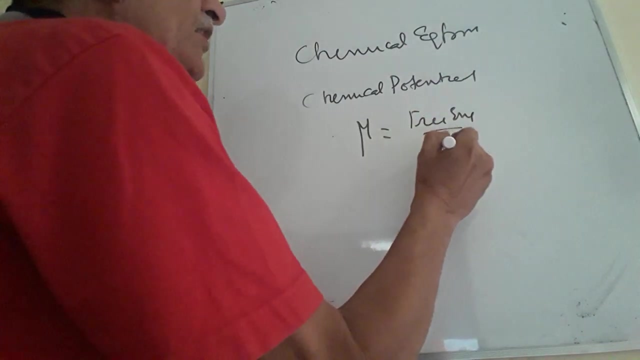 So we have defined a new parameter called chemical potential, Chemical potential Potential. This is given by mu. This is nothing but your free energy per Free energy per mole. Free energy per mole. So another name for free energy per mole is chemical potential. 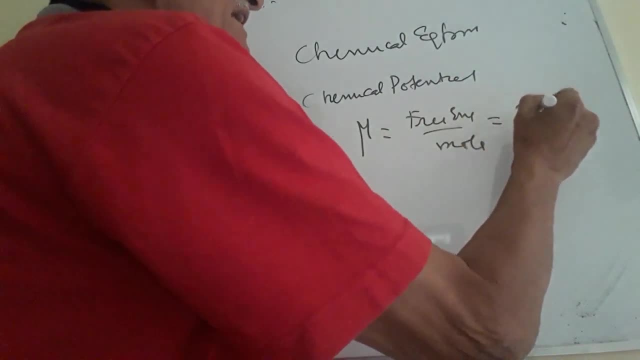 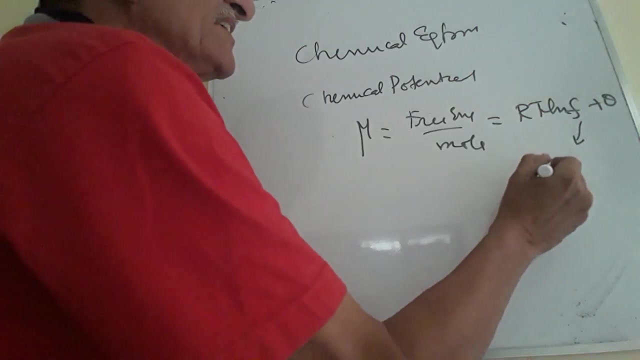 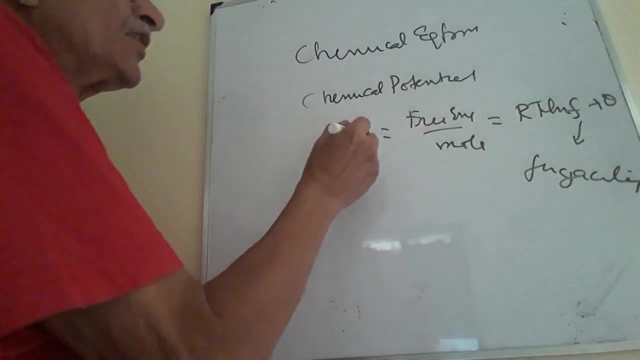 Okay, This is as equal to RT, LNF plus theta. Now this is chemical potential. F is called fugacity, Fugacity, R is gas, T is temperature. Theta is a function of temperature. only This is called chemical potential. 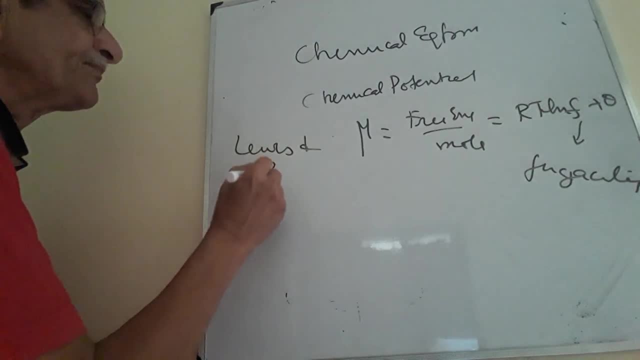 This is called mu And Rantau, Rantau, Rantau Rute. So this is chemical potential. It is called Lewis and Rantau Rute. Now this chemical potential is used in our phase equilibrium. 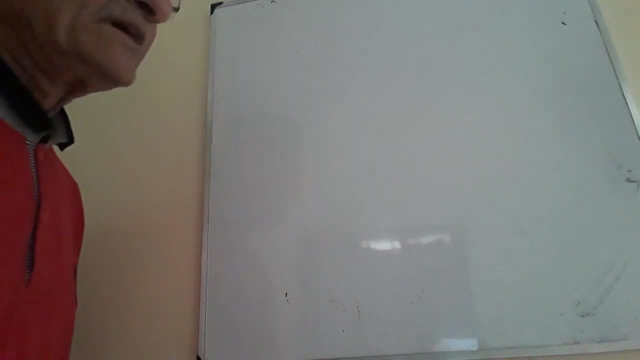 Okay, Phase equilibrium. For example, we have got a liquid phase and a vapor phase. Okay, Liquid phase and vapor phase. If there is vapor here, there is liquid here, Now at equilibrium, the temperature of this phase and this phase will be same. 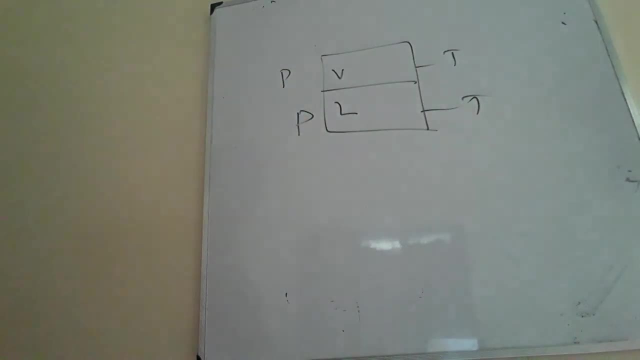 Pressure of this phase and pressure of this phase will be same, So pressure in the vapor phase and liquid phase will be same. pressure will be same. Then, apart from that, we have got chemical equilibrium. What does it say? Suppose we call the chemical potential of the vapor phase? 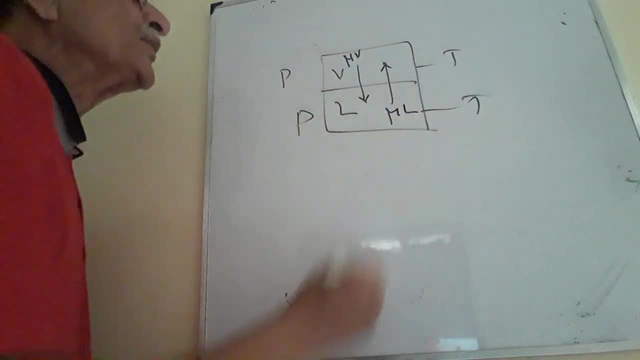 as mu V and chemical potential liquid phase is mu L. Now, at phase equilibrium, apart from pressure equality and temperature equality, we have got chemical potential mu L equal to mu V. That means the chemical potential of liquid phase will be equal to vapor phase. 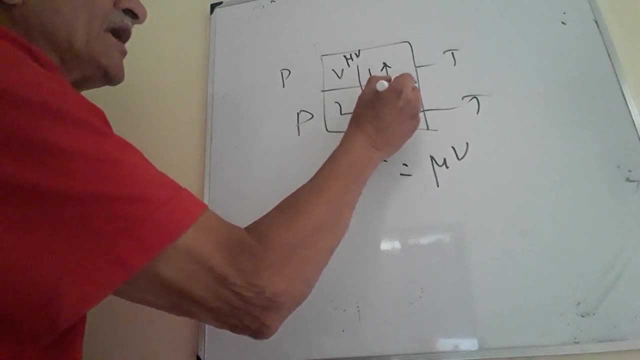 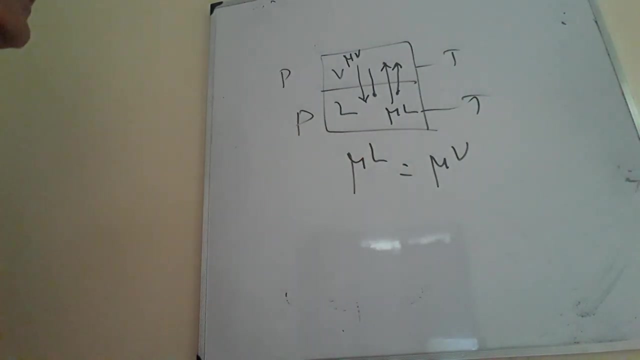 What does it mean If one molecule of the vapor comes to liquid, another molecule go out, like that? Now we are maintaining the equilibrium, So mu L equal to mu V. So for phase equilibrium we have got three parameters: equality of pressure, equality of temperature. 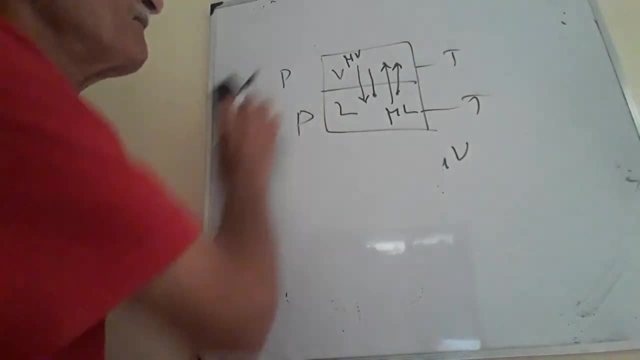 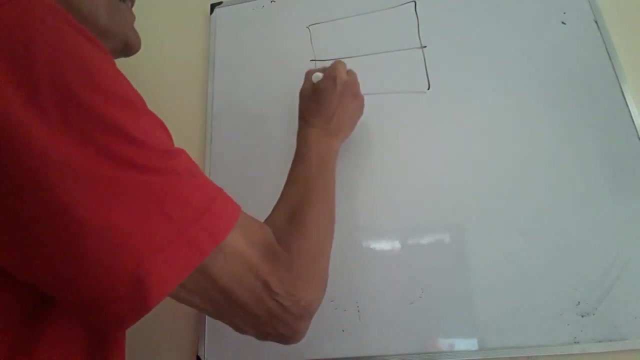 and equality of chemical potential. Now, before going further, we have got two phases here. I am going to say two phase system, two phase, a liquid phase and vapor phase, vapor phase. We can have binary system, two components, terminal system, two, three. 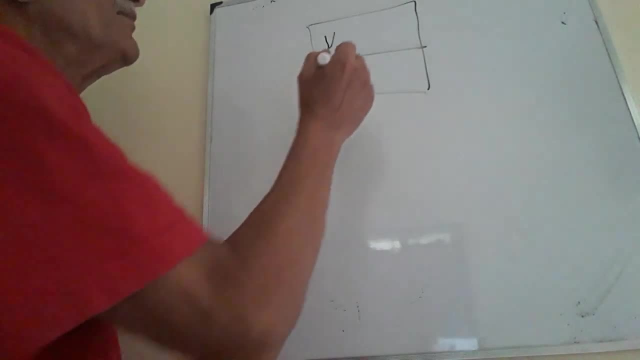 components, etcetera. Now we have seen that at chemical equilibrium, apart from temperature and pressure, the vapor phase chemical potential is equal to vapor phase, liquid phase. Now suppose there are number of components. there are number of components, let us say two binary. 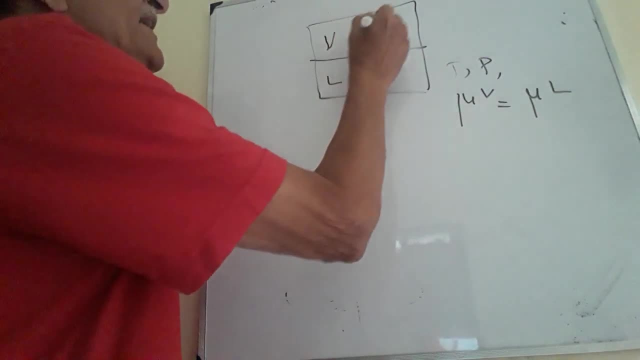 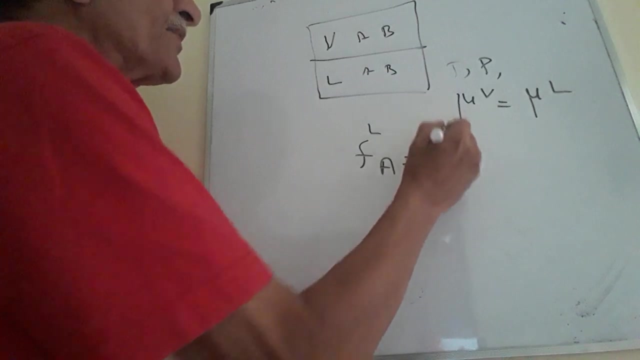 here We have got A and B, liquid phase A and B- vapor phase. Now at equilibrium we have defined this as equal to RT, LNF plus theta. Now, at equilibrium, the liquid phase component A will be equal to vapor phase component A. That is the fugacity of the liquid phase. 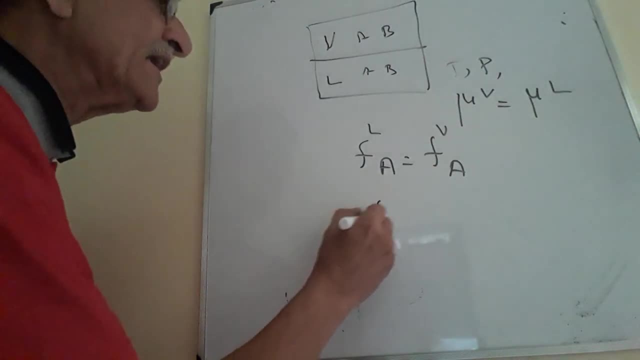 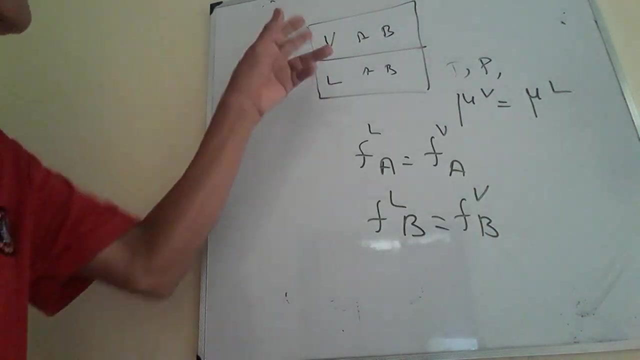 and vapor phase of the component A will be same. Similarly, fugacity of liquid B component B and fugacity of component B in the vapor phase will be same. Now, this is also another criteria, Apart from equal to the chemical potential, the fugacity is liquid phase, vapor phase will be same and this liquid phase Now it has- I am not going in depth into this- At low pressures, at low pressures, it is fugacity equal to pressure F, equal to P at low pressures. at low pressures, See and your distillation. 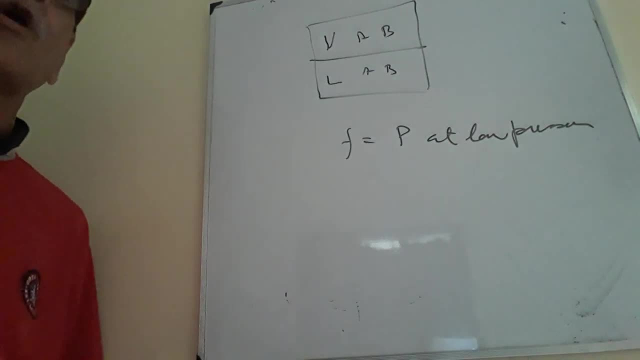 column. now we are going to study male distillation. Distillation columns operate only at massive pressure. Most of the all distillation columns are up to the pressure At massive pressure is low pressure. only In that case fugacity will be equal to pressure. and if the pressure 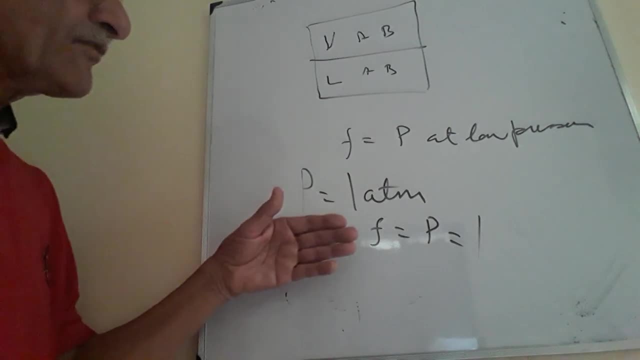 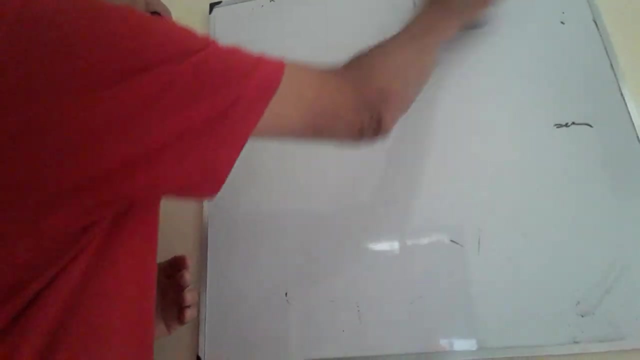 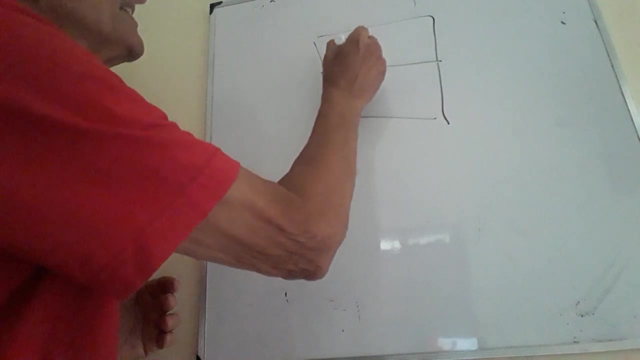 is 1 atmosphere, it will be equal to 1.. So fugacity also has a units of pressure atmosphere. Therefore, at low pressures fugacity is equal to pressure. Now, with this basic understanding, let us look at the vapor phase and liquid phase. We have got vapor phase and liquid. 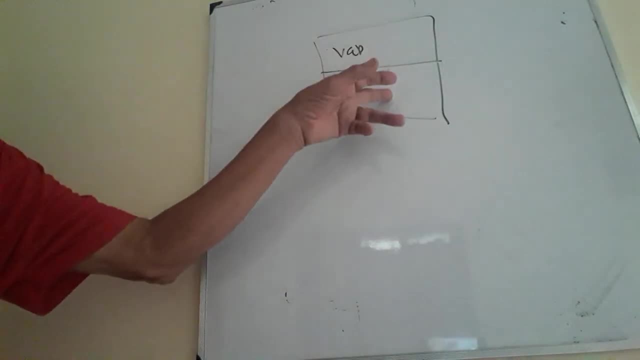 phase. This is vapor, this is liquid, This, of course. of course you can consider this vapor as a gas. What is vapor? is nothing but a condensable gas. it is called vapor. So vapor phase is a liquid phase. Vapor phase: essentially atmospheric pressure- ok, Essentially atmospheric. 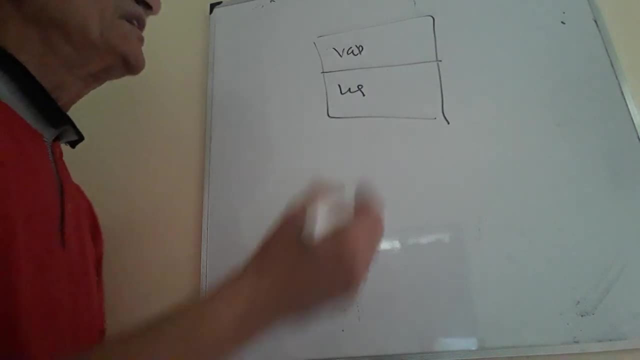 pressure At, essentially at atmospheric pressure. you can apply the ideal gas law, For you have got component A and component B, And for ideal gas law you have got P A equal to N, A into R, T right P A into V ok N A R. 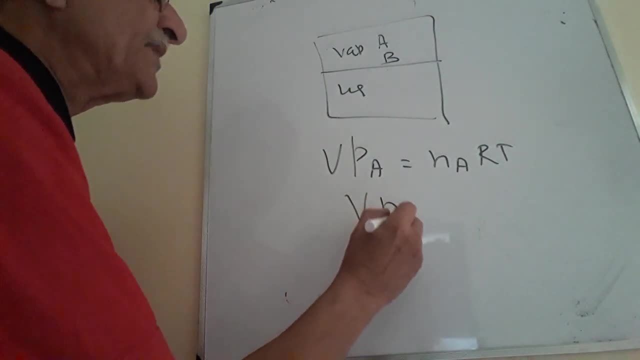 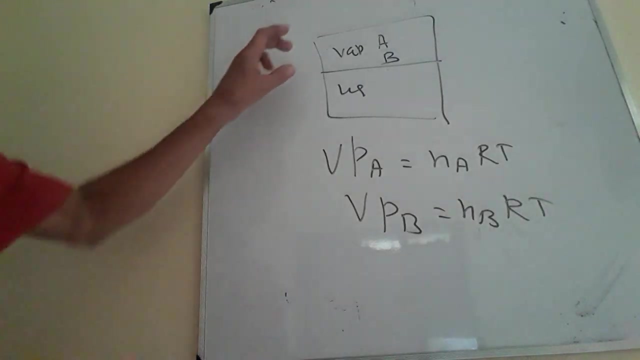 rt. Similarly for b into pb, where pb is a partial pressure of a in the weber phase, nb into rt. So this is the volume of the weber phase: pa is a partial pressure of a and pb is a partial pressure of a and rt. This is Heidelberg's law, Or you know. 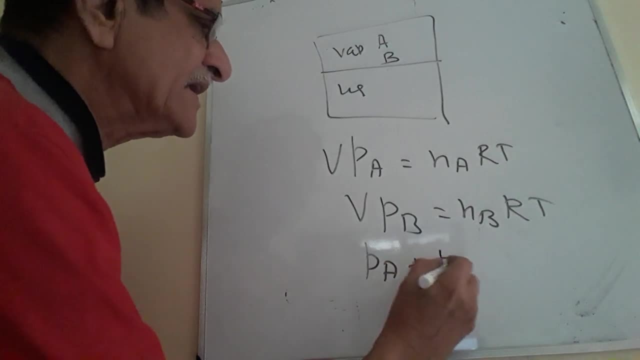 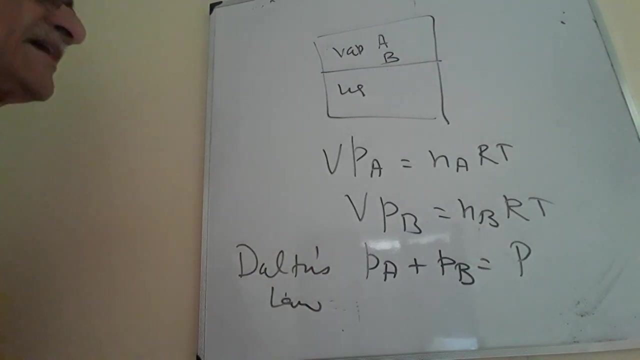 according to D'Arten's law, pa plus pb equal to p. This is D'Arten's law. D'Arten's law says that some of the partial pressures equal to total pressure- okay, and pa equal to rt by v and nb by v into rt- okay. This is the D'Arten's law. So weber phase is: 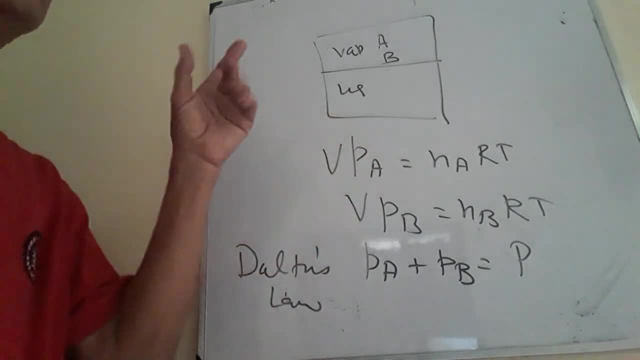 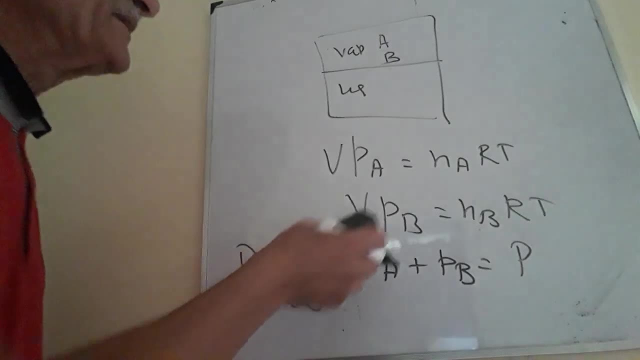 always an ideal gas. Therefore, you can easily apply ideal gas law for each component in the weber phase. There are 10 components. Each one you can apply the weber phase, this one, D'Arten's law. Now coming to look at phase. 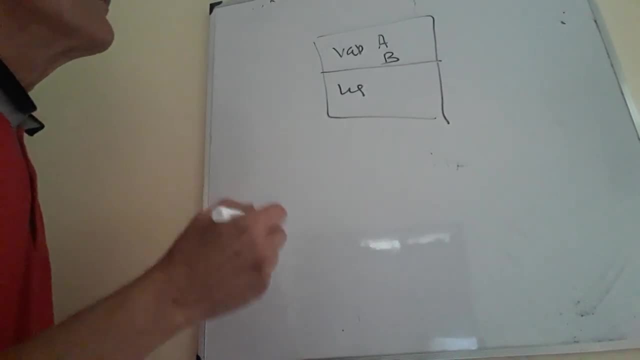 now in weber phase again. you know we have got ideal gas law, That is pb equal to rt. If gas is not ideal, what you do is we use the EZ factor. EZ is called the compression factor, So ideal gas law, EZ equal to 1.. If the gas behaves ideally, EZ. 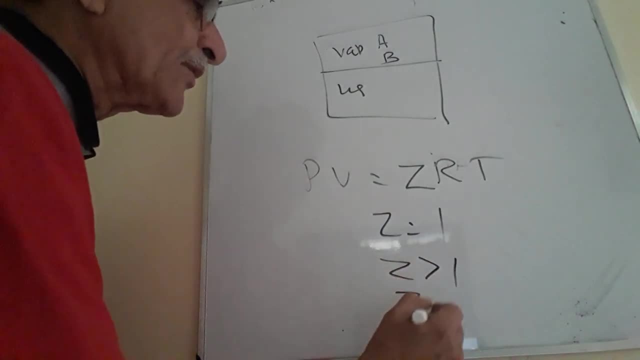 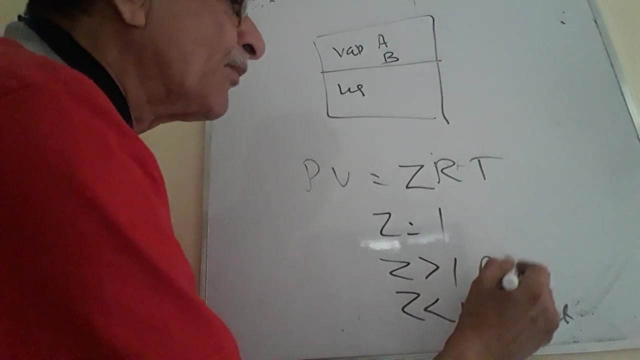 equal to 1.. If EZ can be greater than 1 or EZ can be less than 1.. If the attractive forces are very important, then EZ is less than 1.. If the repulsive forces between the molecules are important, then EZ is less than 1.. If the repulsive forces between the molecules 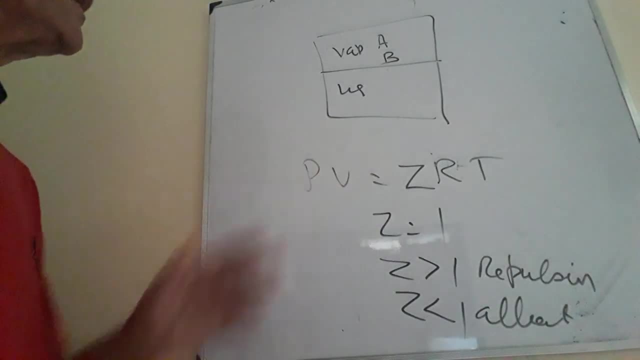 are important than 1, so eZ is less than 1.. But in our case EZ is equal to 1.. Compressive factors: measures of deviation from idle gas behavior. Since the weber phase is going to be ideal gas, we use EZ equal to 1 for the weber phase. No problem at all. Now coming 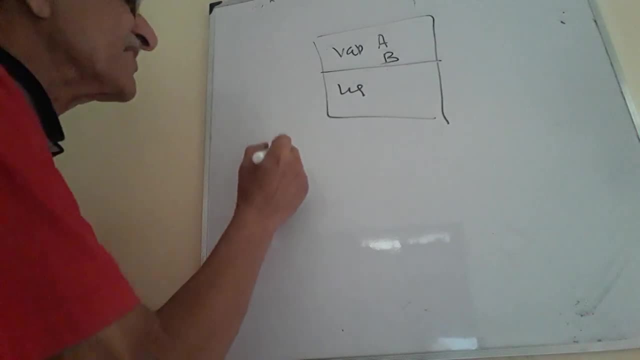 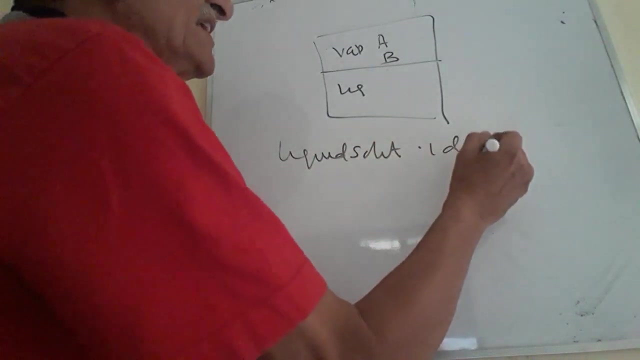 to liquid phase. liquid solution Here. you got this aqui solution, So liquid solutions we can apply. we have got ideal solutions. some books call it per buyer material, we call it per customer, We call this per year than per bacteria Of those one from each. 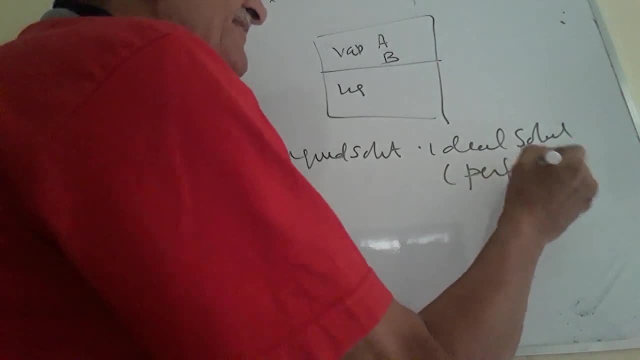 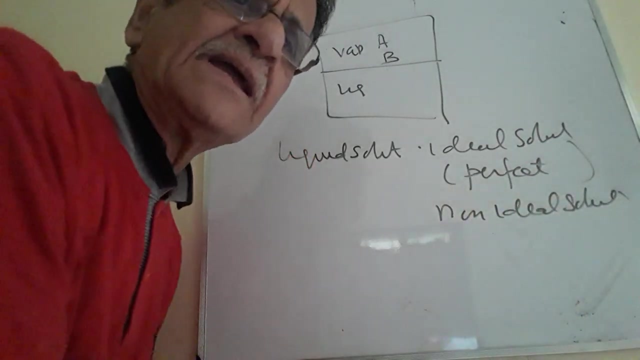 See, you see this. this is for every case. you say: object of the previous phase, wafer, So Perfect solution. because not to confuse with ideal gas, okay, and non-ideal solution, non-ideal solution, this is called imperfect gas, imperfect gas, imperfect solution. another name is imperfect. 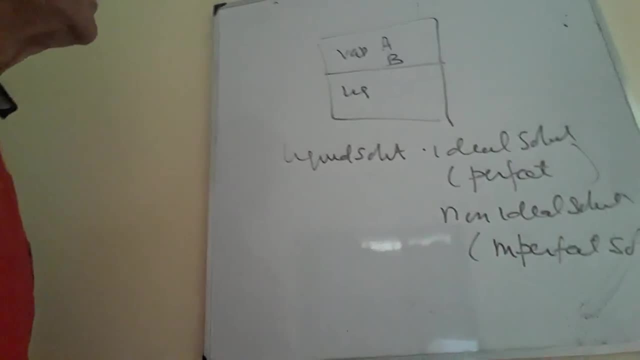 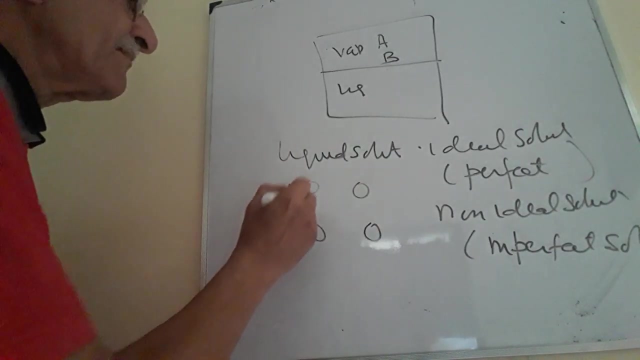 solution. Now for a perfect solution. okay, what is the ideal solution? We have got two components: A and B, A and B. this is A, this is B. Now, according to ideal solution, the force of attraction or repulsivity: A, A and A, and. 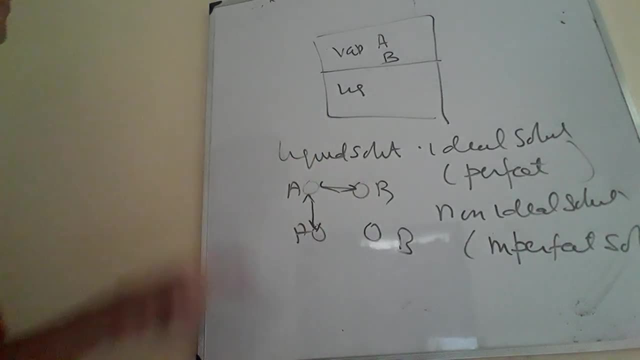 A and B will be of the same order. If the A and A is 1 newton, A and B also 1 newton, that means forces like forces between like molecules and unlike molecules are exactly same. In that case it is the ideal solution. 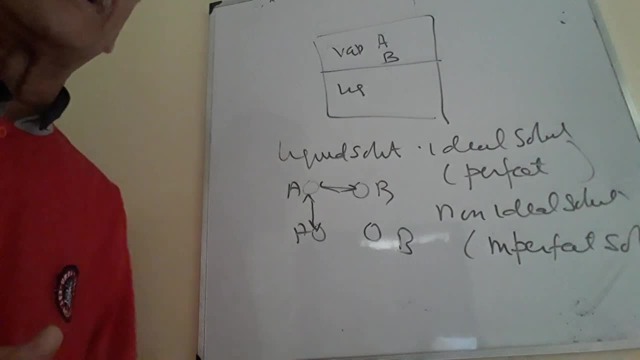 For example, you take benzene, toluene just next to the aromatic series, so we have methane, ethane next to the aromatic series. those things always behave ideal solutions. So this is ideal For non-ideal solutions. it is there will be attractive force. 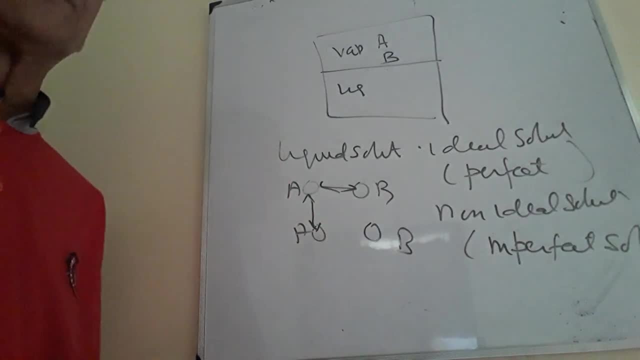 For example, you put water and sulfuric acid, temperature will be, heating will be there. If you put potassium hydroxide in liquid water, cooling will be there, Whereas for ideal solution you put, there is no change in temperature. 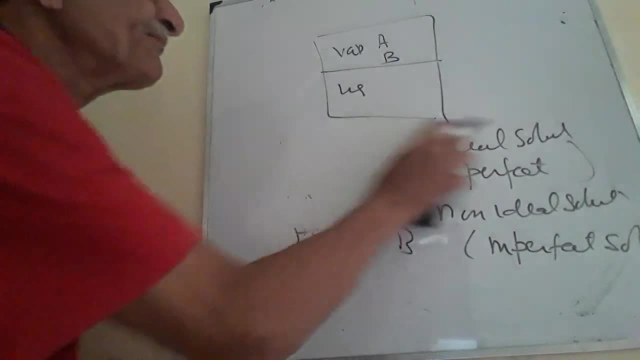 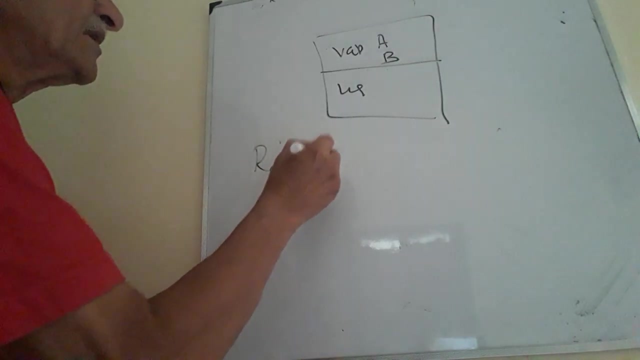 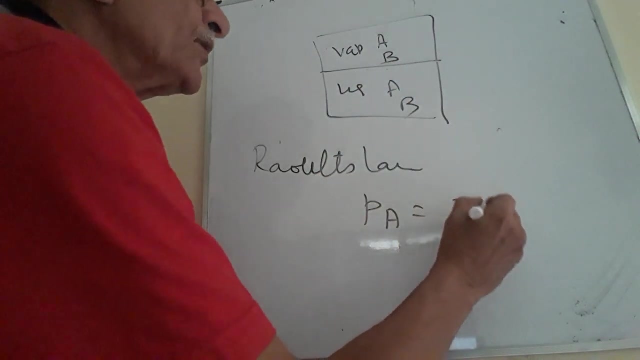 Therefore, ideal solution is not always possible. Most of the cases it is a non-ideal solution, And for ideal solutions we use Raoult's law. Raoult's law, So for A and B is there. Then positive fraction of A is equal to X. A into P, A prime. 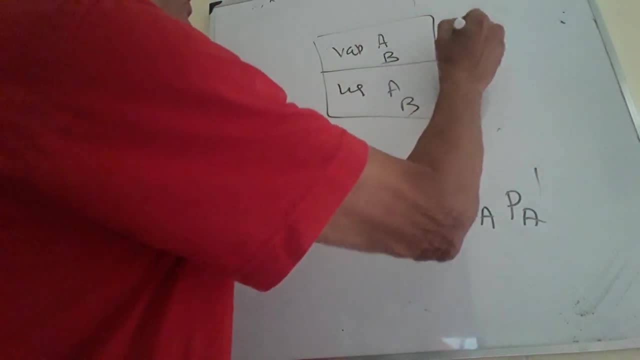 See Y you have used here. we can use here: P A equal to Y A into P. Positive fraction of A in the vapor phase is and P B equal to Y B into P, Where Y A is the mole fraction of A in the vapor phase. 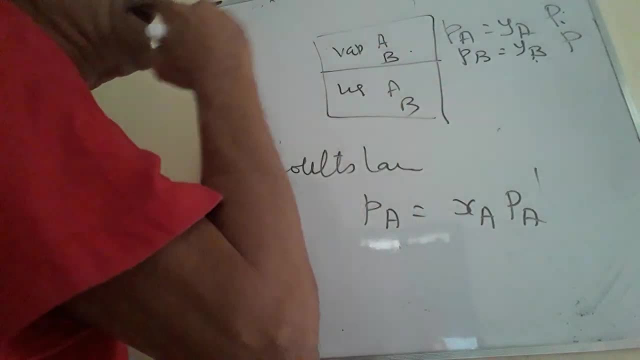 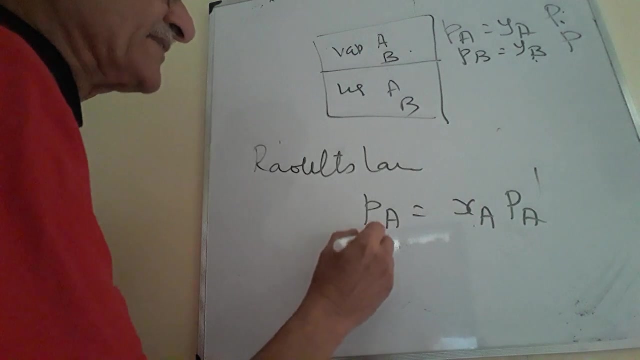 Why it stands for vapor phase Y. B is the mole fraction of B in the vapor phase And P A plus P B equal to P. Similarly, in liquid phase X A is the mole fraction of liquid. in liquid phase, P A is the vapor pressure at the temperature. 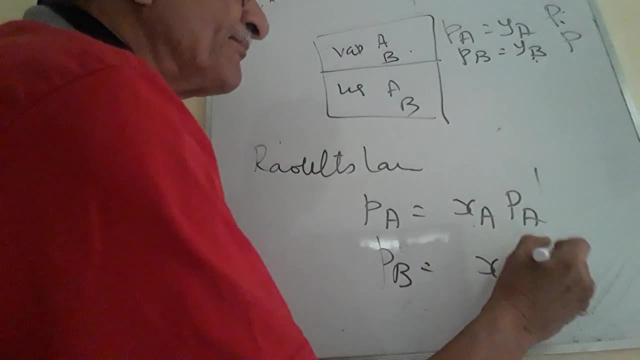 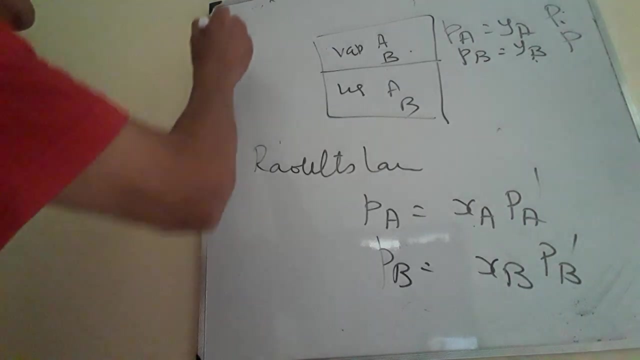 P B is equal to X A, X B into P B prime. P B prime is nothing but a vapor. P A prime, P B prime are vapor pressure at the temperature. Okay, We can use Cox plot. You know, you got a Cox plot. 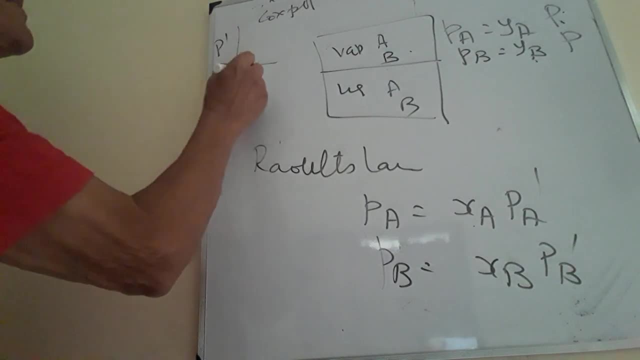 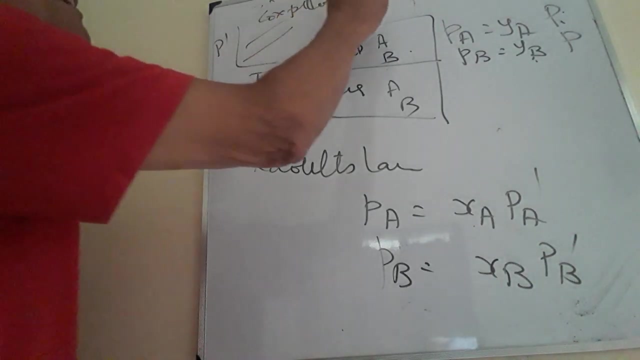 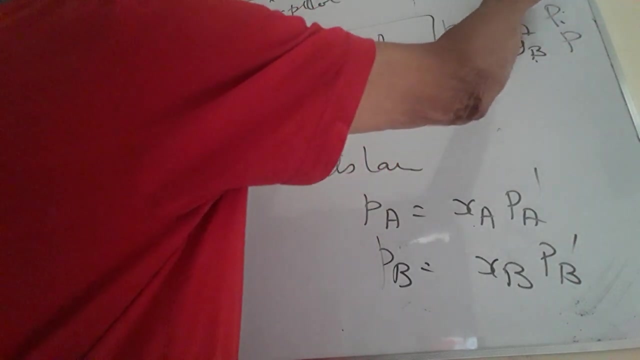 Which gives for different temperature: vapor pressure versus temperature For many substances. that will be in the Cox plot. Or you can use Anton equation. Now: P prime equal to A plus B by C plus That is T, Because T is the temperature. 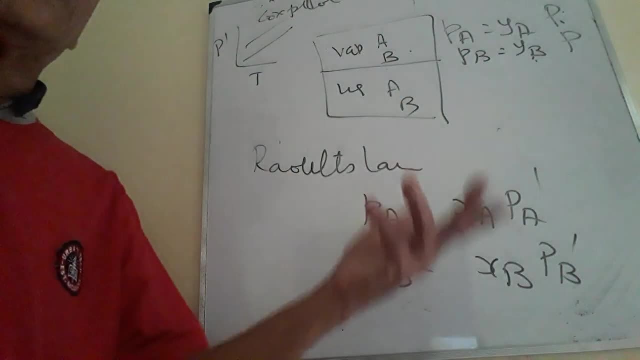 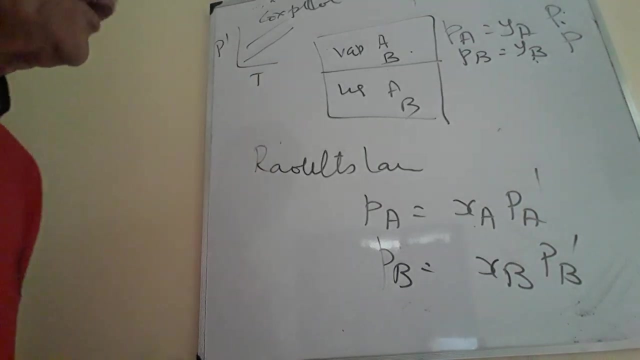 C. A, B, C are constants And this constant A, B and C are available for many substances in any literature. You take Hara, equilibrium, thermodynamics Or this Cox plot also you can use Now for ideal solution. we use this. 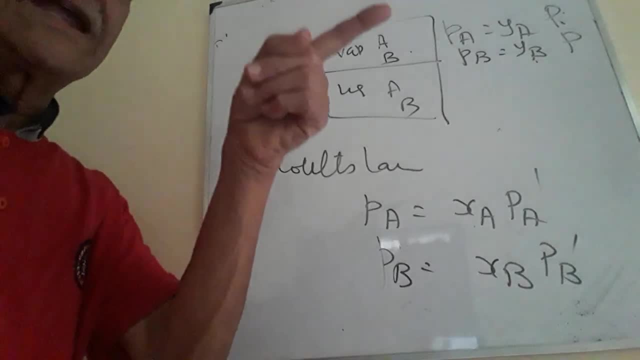 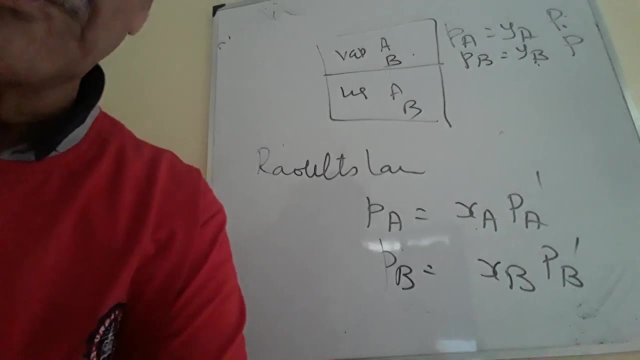 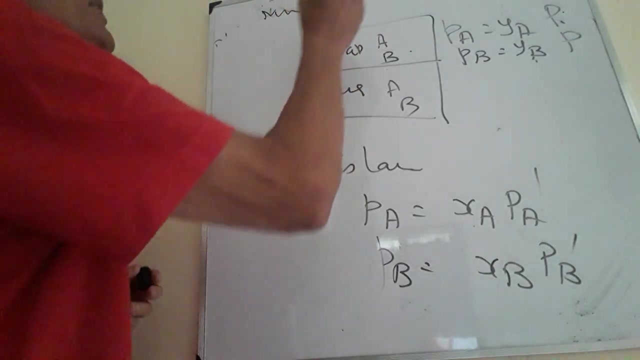 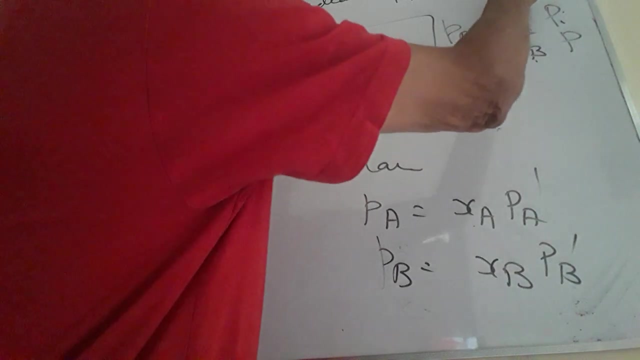 For non-ideal solution, we introduce the fact that, just like is it for ideal gases, non-ideal gas We can use for non-ideal solution- non-ideal For non-ideal liquid, Non-ideal Ideal liquid solutions, we use what is called as P A equal to gamma A, X A, P A prime. 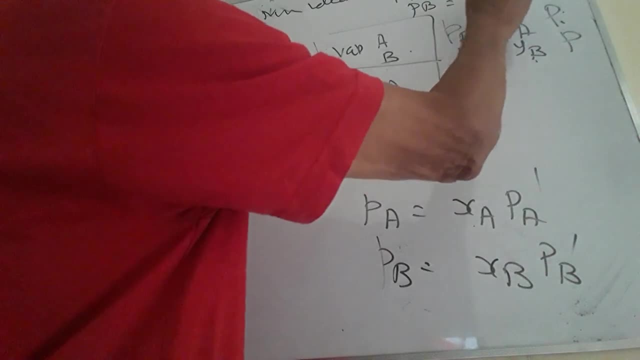 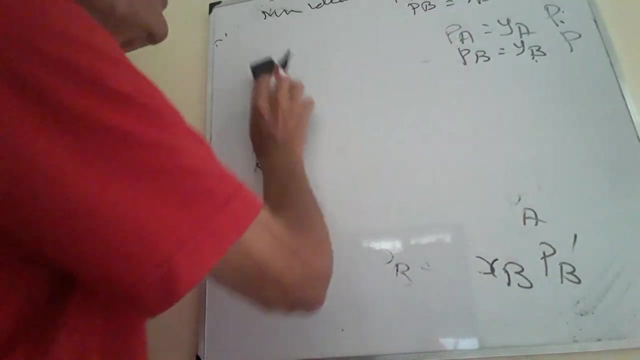 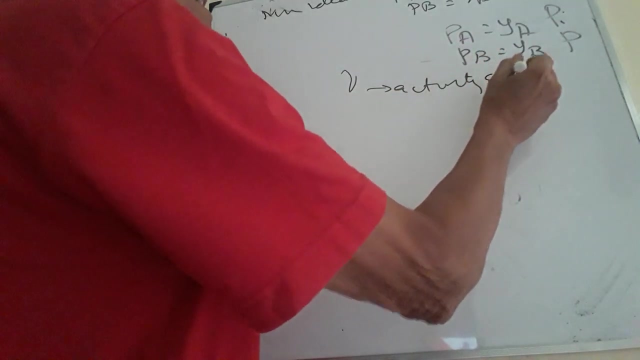 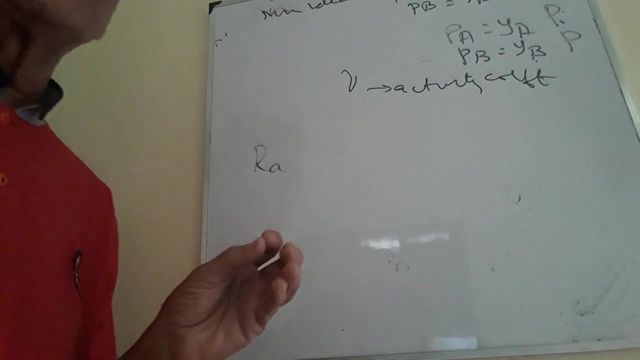 And P B equal to gamma B, X B, P B prime. The gamma is called the activity coefficient. Activity coefficient Gamma is called activity coefficient Gamma A and Gamma B. So it's a measure of deviation from ideal solution behaviour, Just as is it. it's a measure of deviation from ideal gas behaviour. 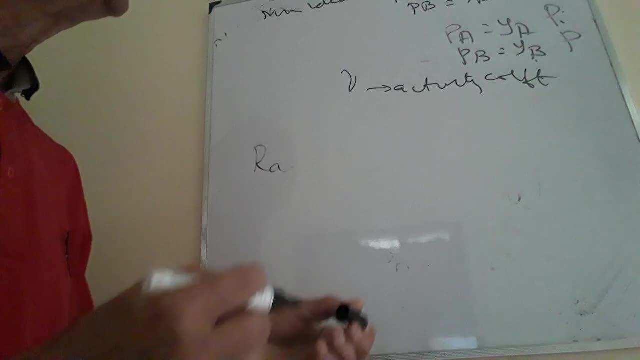 gamma A and gamma B are measures of deviation from ideal solution behaviour. If Gamma is 1, it is an ideal solution. This Gamma A and Gamma B can calculate from Bandler equation, Margus equation, Mule's equation. 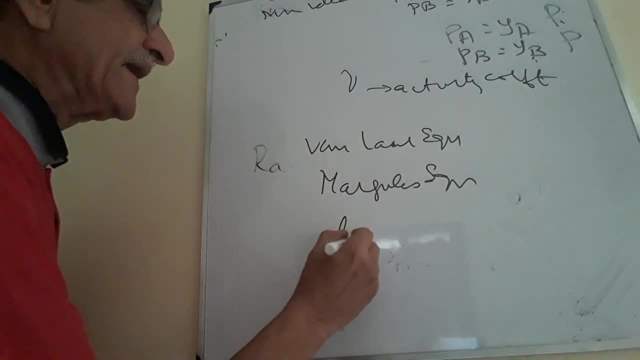 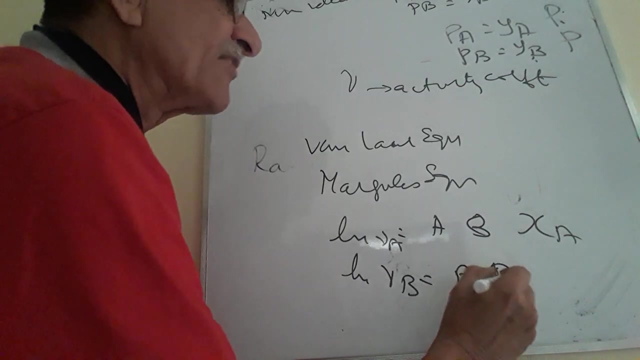 Mules equation. equation relate log gamma A as some function of A, B and composition C x. Similarly, log gamma B is equal to. it is a function of A, B and index B. These equations are available in literature. Once you know the constant A and B and C, you can calculate log gamma. 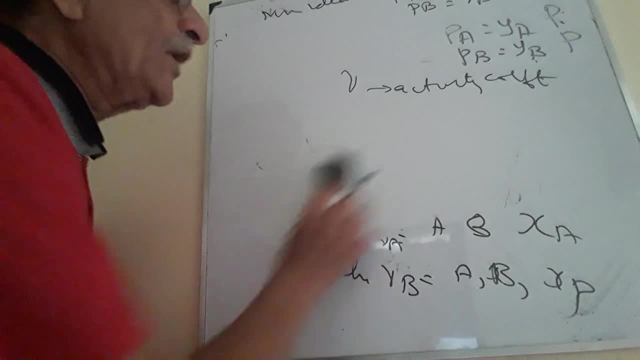 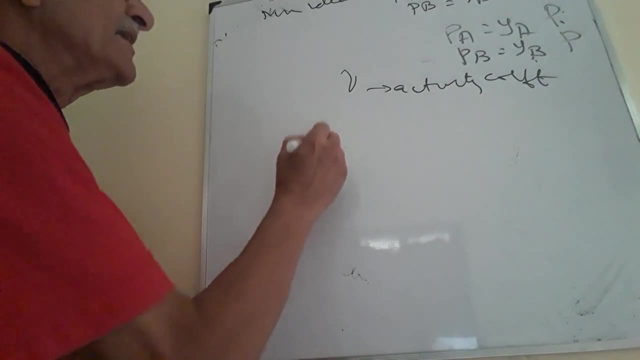 A and gamma B, So you can use the gamma A there and gamma B Now at equilibrium. I told you fugacity, and fugacity is same as pressure. Then we can say vapor pressure of the vapor phase, P A in vapor phase is equal to P A in liquid phase. Similarly, P. 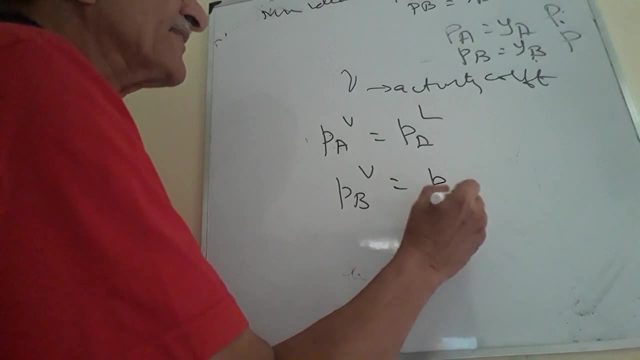 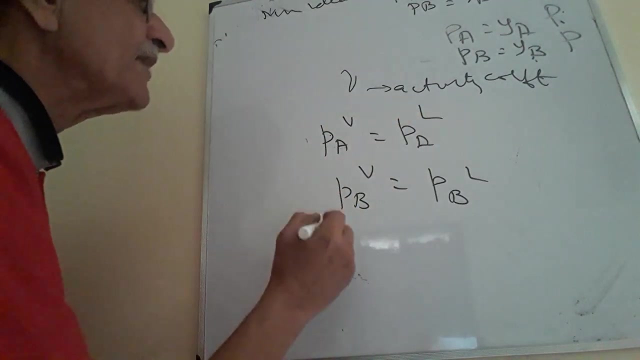 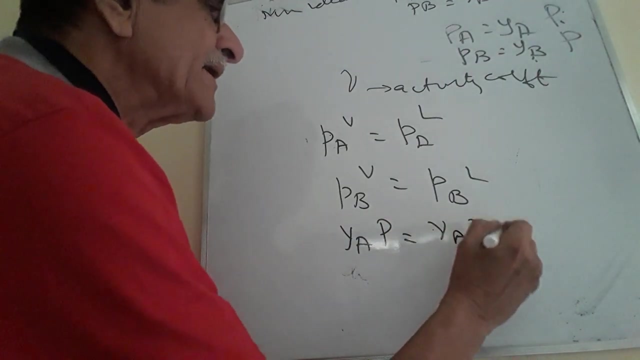 B in the vapor phase is equal to P B in the liquid phase. Now we can write: P A equal to: this is vapor. this is liquid. Now P A in the vapor phase is y A into P. this is equal to gamma A, x A, P A prime. 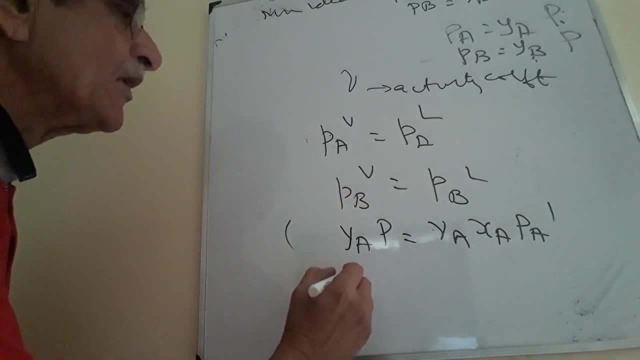 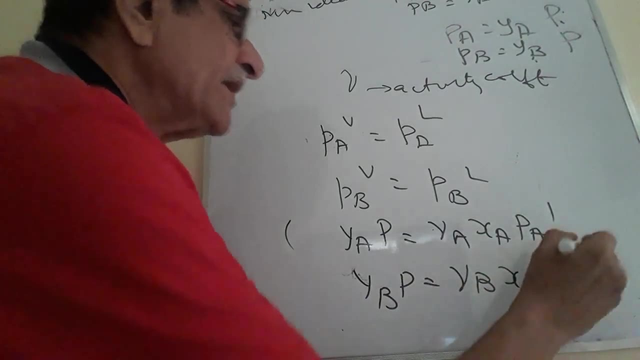 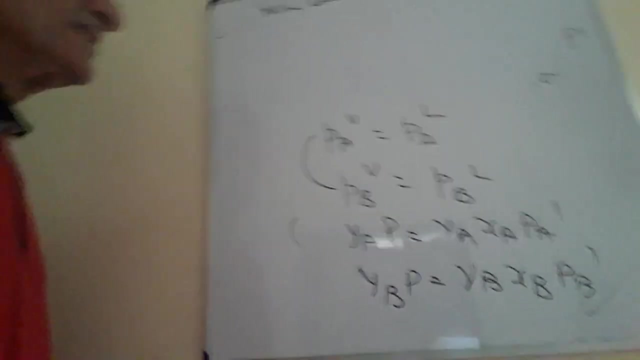 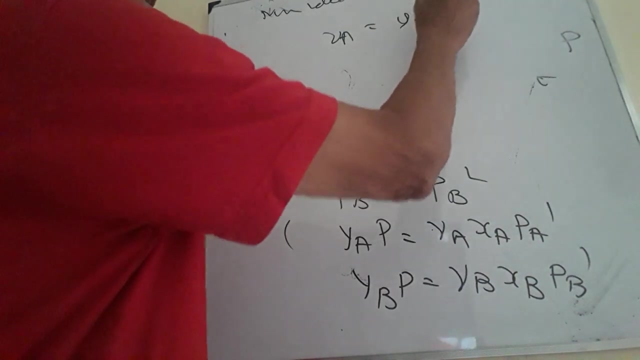 And for this you can write: y B into P is equal to gamma B, x B into P, B prime. And we have seen that at equilibrium this will be same because fugacity and pressure are same. So from there you can write gamma A equal to y A into P by x A into P, A prime. Then gamma B is equal to y A into P by x A into P A prime. Then gamma B is equal to y A into P by x A into P A prime, And for this you can write: y B into P is equal. 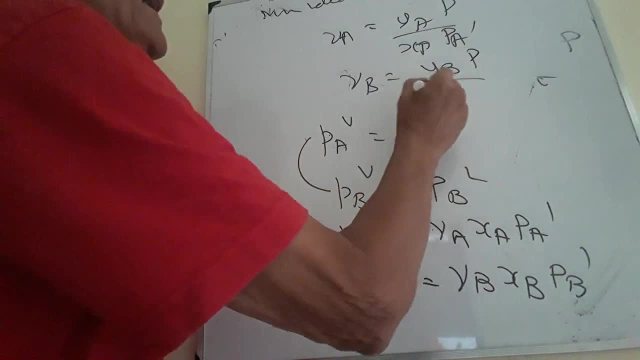 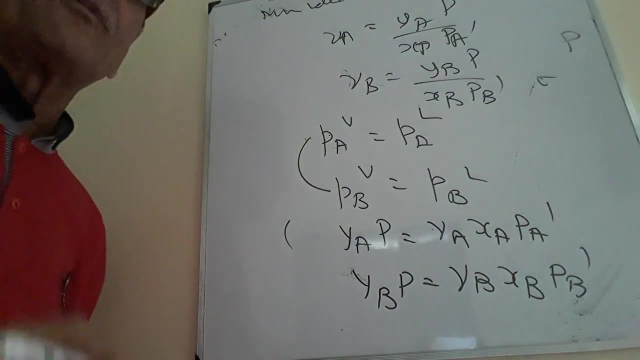 to y, B into P, by x, B into P, B, prime. Now the pressure, total pressure, is known. The distillation column operates at the atmospheric pressure. P is known. Where pressure in each plate, the temperature will change. If you take distillation column, pressure is same. 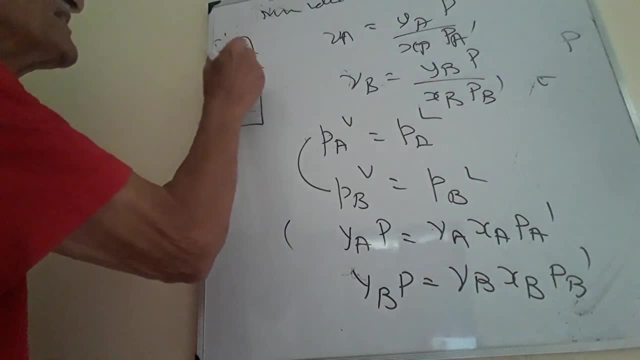 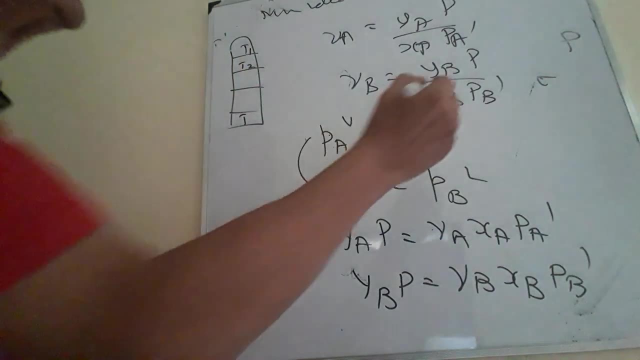 throughout Each plate the temperature will change: T 1, T 2, etc. At the bottom most it will be hottest because it reboils here. Top most is the least. So once you know the temperature in different plates we can calculate x, B, B, prime. So we can write y B into P. 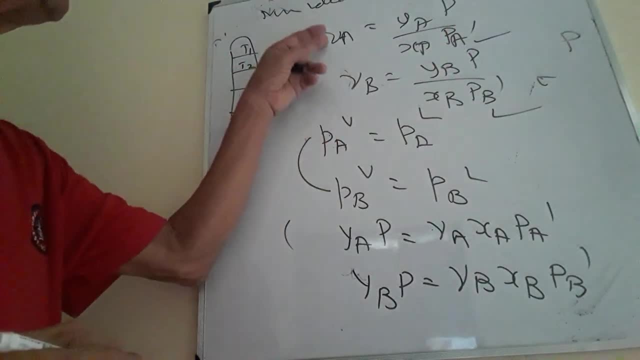 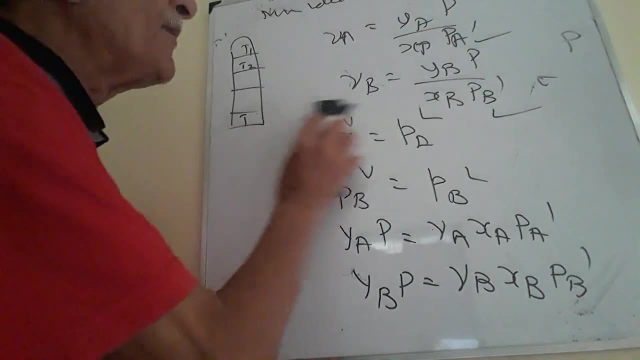 prime. From the Cox plot you can get wave pressure, The gamma B, and gamma B for the substance, whatever it is. you can get it from the Verlander equation, Margarethe equation. Now, based on this, you can calculate the compression: x A and x B, y A and y, y and.